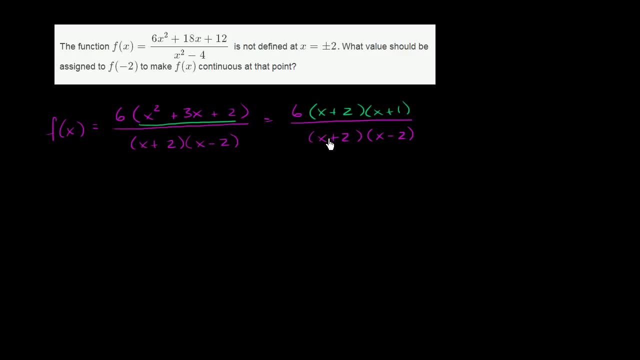 then we can divide both the numerator and the denominator by x plus 2.. The reason why I'm making that constraint is that if x were to be equal to negative 2, then x plus 2 is going to be equal to 0.. 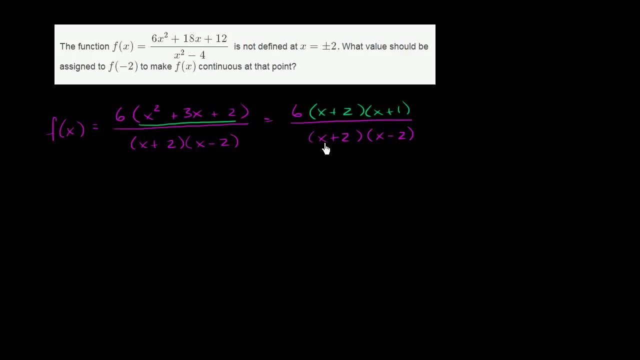 And you won't be able to do that. You can't. We don't know what it means to divide something by 0. So we could say that This is going to be equal to: So we can divide the numerator and the denominator by x plus 2.. 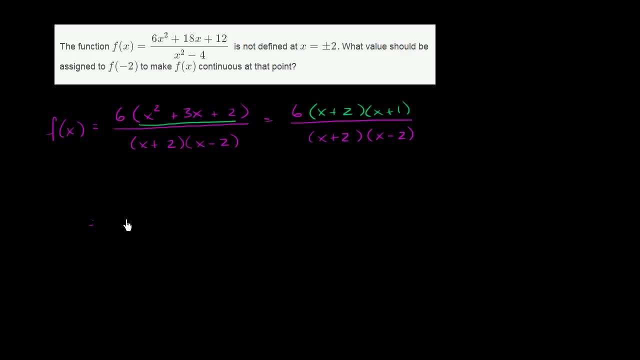 But we have to assume that x is not equal to negative 2.. So this is equal to 6 times. So we're going to divide by x plus 2 in the numerator, x plus 2 in the denominator, So it's going to be 6 times x plus 1 over x minus 2.. 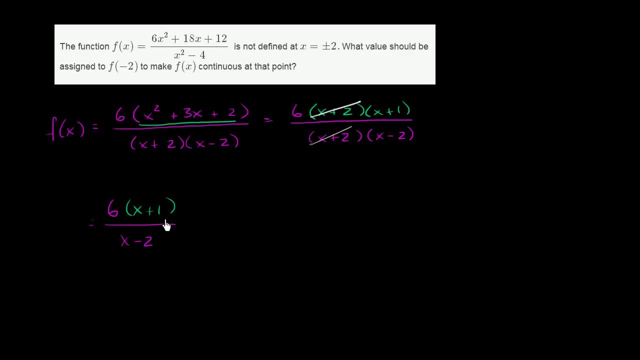 And we have to put the constraint here, because now we've changed it. Now this expression over here is actually defined at x equals negative 2.. But in order to be equivalent to the original function we have to constrain it. So we will say for x not equal to negative 2.. 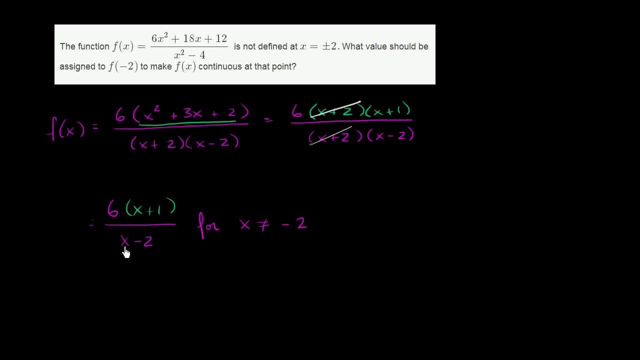 And it's also obvious that x can't be equal to 2 here. This one also isn't defined at positive 2 because you're dividing by 0. So you could say, for x does not equal to positive or negative 2, if you want to make it very explicit. 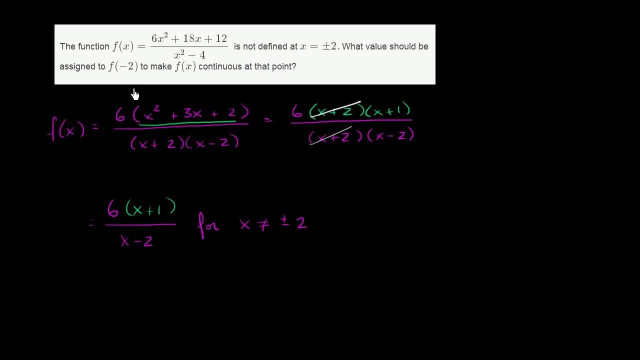 But they ask us: what can we assign f of negative 2 to make the function continuous at the point? Well, the function is completely equivalent to this expression, except that the function is not defined at x equals negative 2.. So that's why we had to put that constraint here. 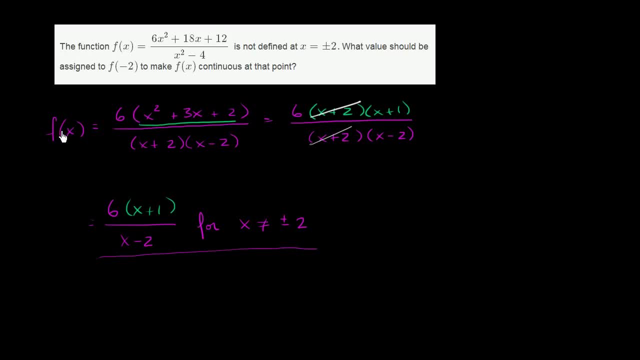 if we wanted this to be the same thing as our original function, But if we wanted to re-engineer the function so it is continuous at that point, well then we just have to set f of x equal to whatever this expression would have been when x is equal to negative 2.. 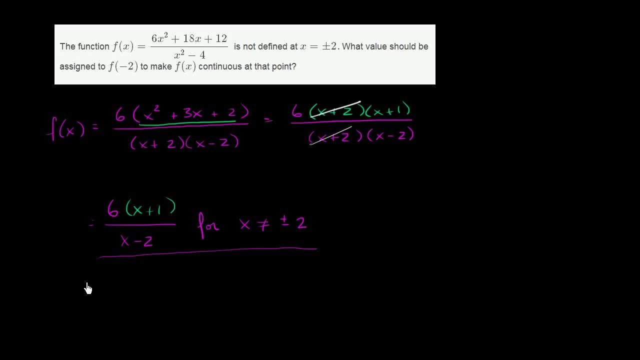 So let's think about that. So 6 times negative, 2 plus 1 over negative 2 minus 2 is equal to this is 6 times negative 1, so it's negative 6, over negative 4, which is equal to 3 halves.